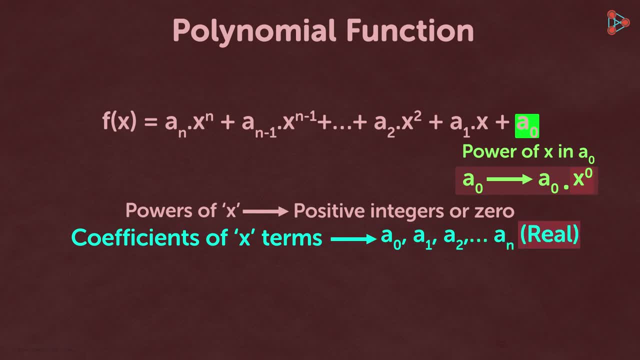 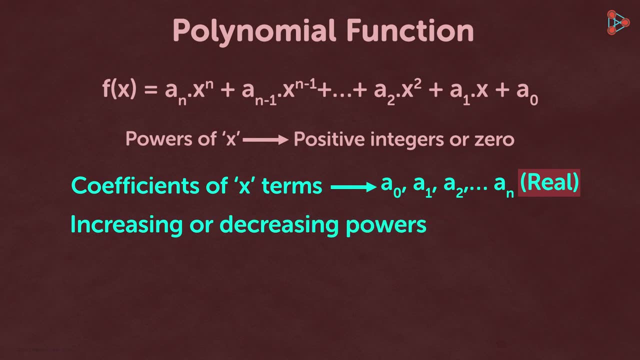 These are all terms of x. So what is the power of x in the term a zero? These are all real coefficients. Now in what order do we write the terms? Should the terms be written in increasing or decreasing powers of x? Both the ways are mathematically correct, since they result in the same function. 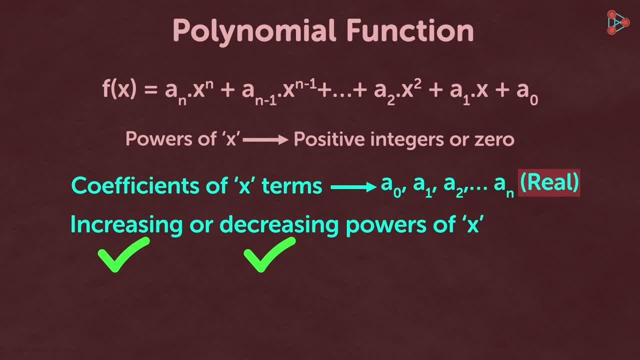 In our video we have chosen to write the function in the order of decreasing powers of x. Writing the terms in descending order of power is called the standard form. Now, what's the degree of a polynomial function? We can write it in the order of decreasing powers of x. 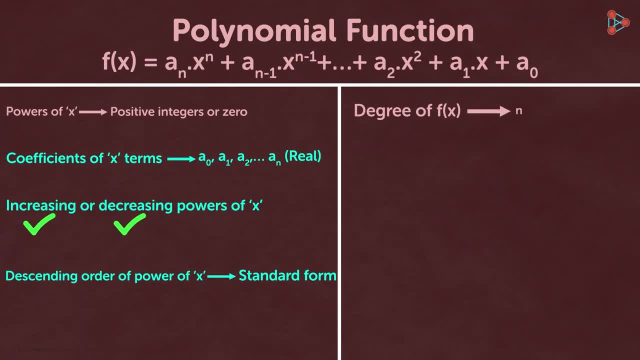 Now, what is a function of x? Can we say that the degree of a function is n? This happens when the highest power of x is n and the coefficient of x raised to n, a n is not equal to zero. What happens when a? n is equal to zero? 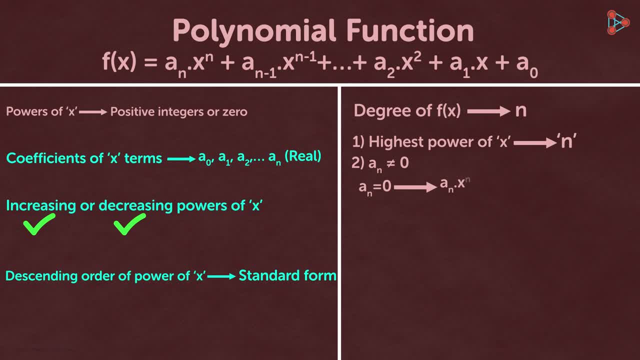 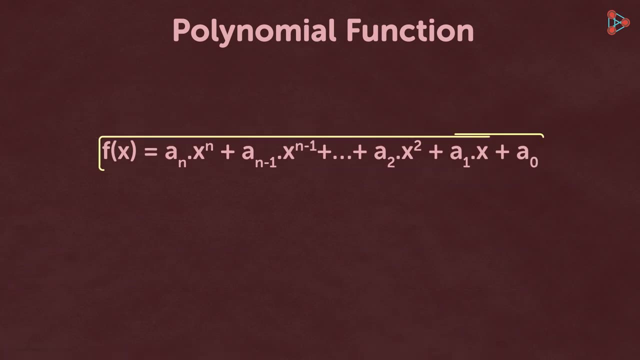 Then the term a, n multiplied by x, raised to n, would be zero, making the degree of the polynomial n minus one. So we know what the degree of a polynomial function is polynomial is. Now we look closely at the terms to understand the anatomy of our polynomial function. 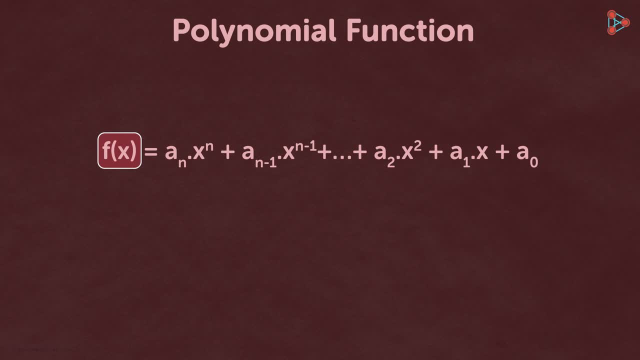 Here is our polynomial function: f of x, a. n is the leading coefficient. This is because it is the coefficient of the x term with the highest power, n. Can you guess what the terms a, zero, a, one times x and times x squared are called? 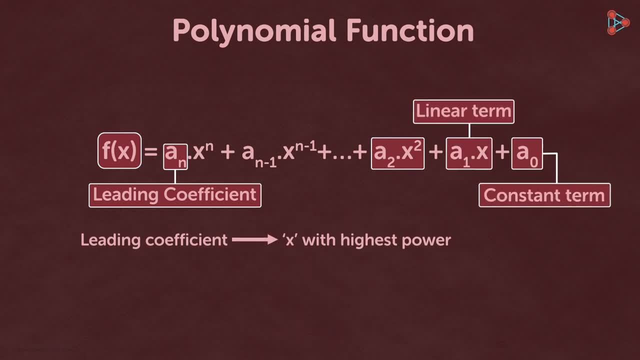 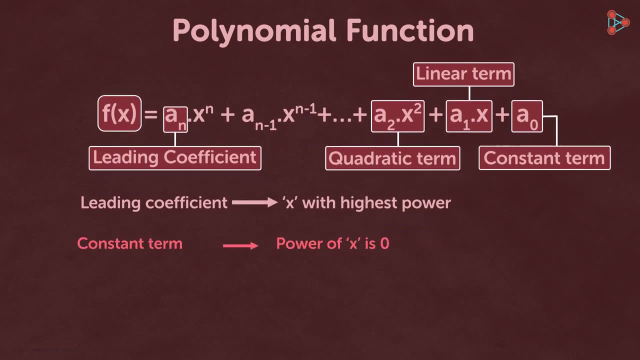 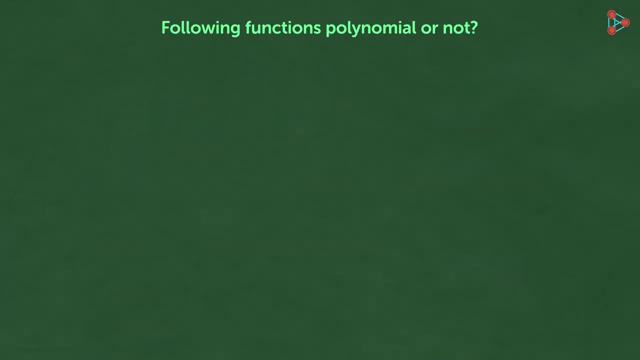 They are called the constant term, the linear term and the quadratic term respectively. This is because the power of x in each of these terms is zero, one and two respectively. Now let us test our understanding to see if the following functions are polynomial functions. 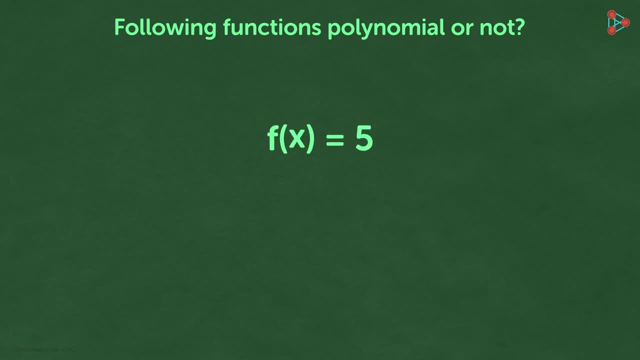 or not? Is f equal to five, a polynomial function? Yes, it is a polynomial function of degree zero. This is because five can be written as five multiplied by x raised to zero. Here, the highest degree of the function is zero. What about these two functions?